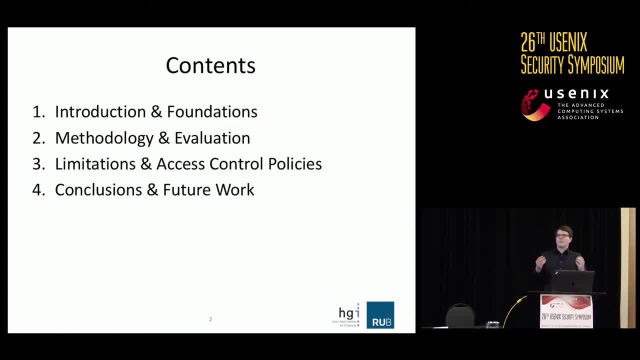 access control policies and whether they match with the same original policy or not. So we will see that. And, last but not least, there is a conclusion part with an outlook and we will discuss some future work. So there's a lot of things to do, but yeah. 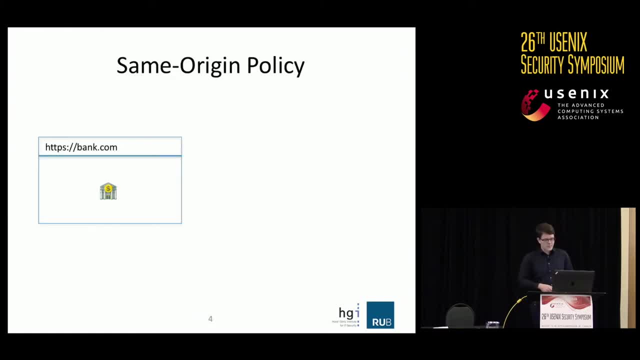 Let's go through the talk. So first of all, the introduction and foundations part. Imagine the following case: We have a website And, for example, in Google Chrome or whatever, And this website is called httpsbankcom And there is loaded some HTML code and CSS. 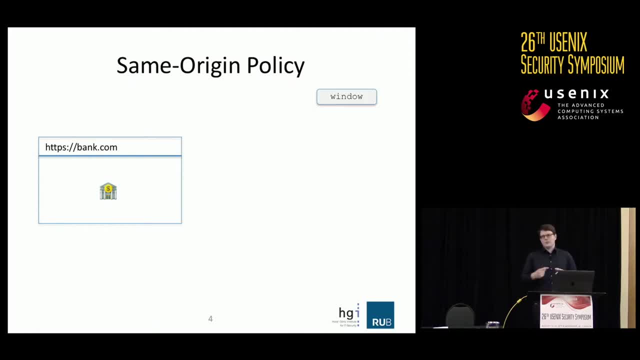 code, JavaScript on whatever. And when we look into the document object model, so the DOM, we can see that depends always on the view. but maybe the root element might be the window And under the window element, or as a child of a window element, we might have document. 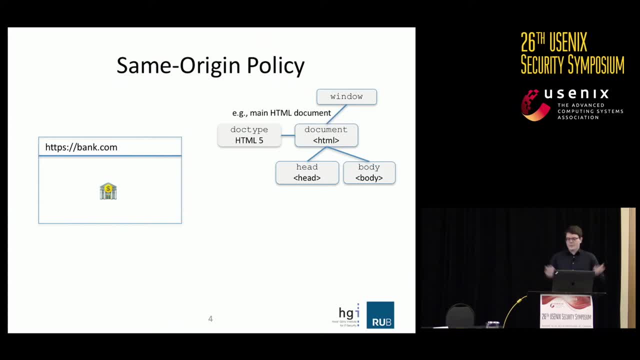 We might have a doc type, an HTML5 doc type, HTML4.01 or whatever, And it had a body. And when we go even deeper, we also have these fragments here. So script, image link and many, many popular things- iFrame, for example. 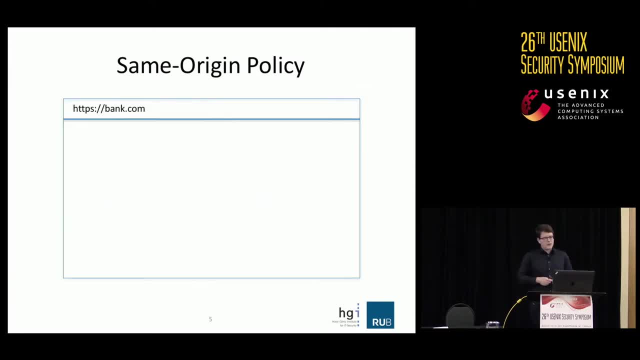 So when we have this scenario here and make it a little bit more complex, there could be something like this: So we have a website with an iFrame, So we have a window and a frame, a subwindow, And this frame here loads also a website. This is the same website with 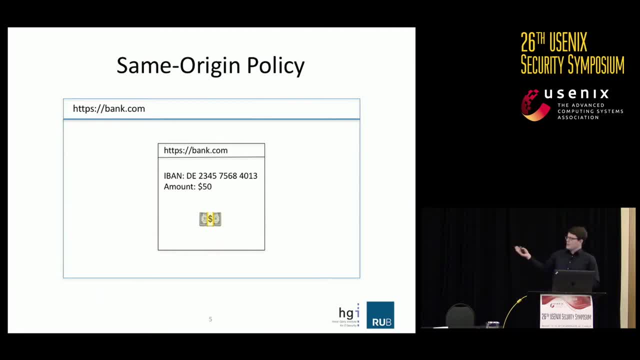 the same origin, bankcom, And we can see that there- oh, it's a small pointer- have an international band account number here and, yeah, also an amount. so we want to transfer 50 bucks to my bank account and an honest party, like a developer from bankcom might say: 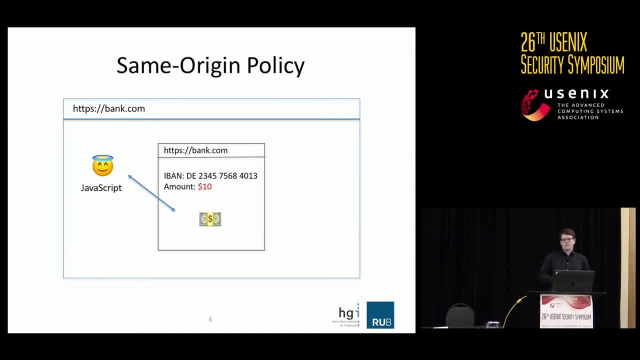 well, let's change the amount to $10. so that is totally fine, because we have act on the same origin. and the question arises: what happens when there is attackersorg? so this guy here is, you see, that attackersorg and he wants to access code or content from bankcom. and in case that this might be possible, 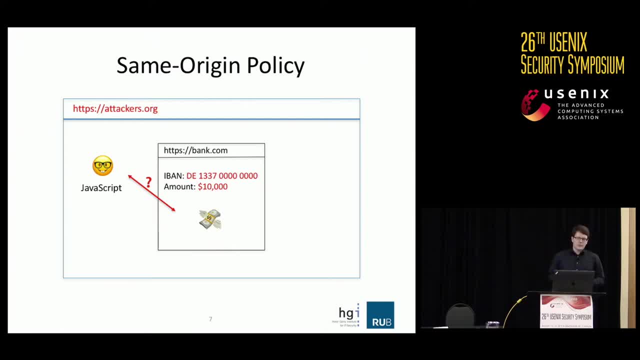 there, when we have a same original policy, bypass this is, of course, hopefully not possible and the same original policy protects us somehow, dependent on different origin aspects like port, protocol and domain. but this is just half of the truth. we have many, many limitations, many exceptions. a well-known one is Internet Explorer, which doesn't care about the 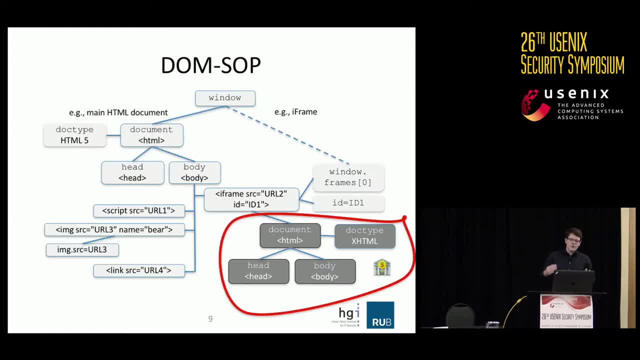 port and so on, and when you go into the DOM- so this is just a small abstract- we can see that there is something like a firewall which is around the DOM of the domain. We have our iframes and this firewall manages well. do you have access or not? 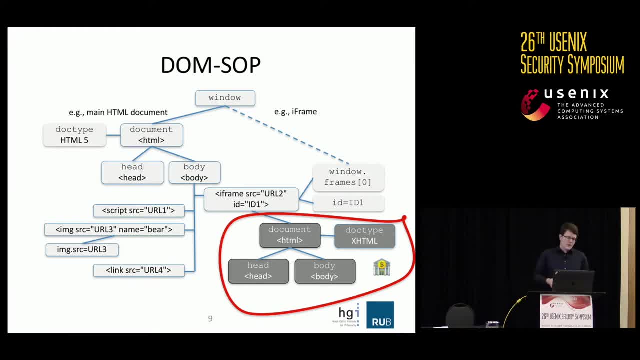 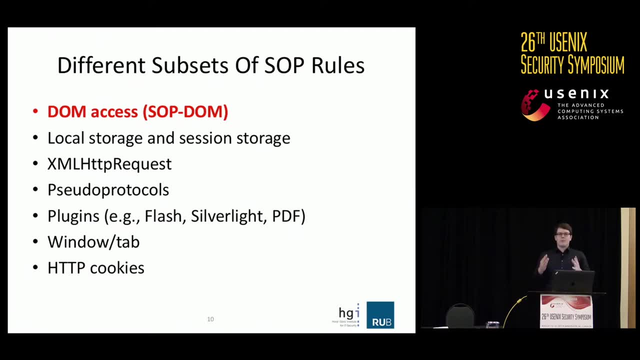 and currently we are talking about the DOM SOP. so this is just a small small subset of the same original policy. Same original policy is actually a set of policies and one subset is the DOM subset. There are also some other well-known policies, like a local storage and 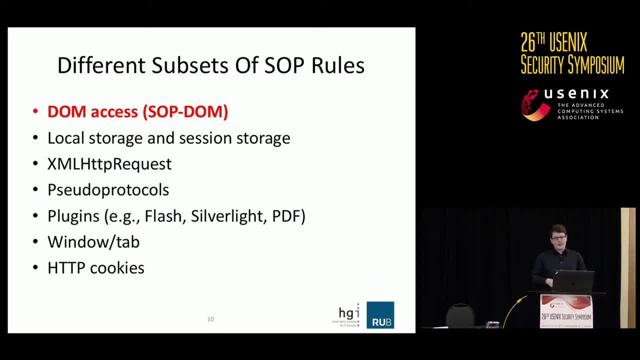 session storage SOP. we have an own SOP for AJAX, for pseudo protocols like a data URIs, JavaScript colon and so on, even for flash, silverlight and PDF. so PDF files have their own same original policy. and when we look on things like window dot opener, we can also say that even a window or a tab has its own SOP. and 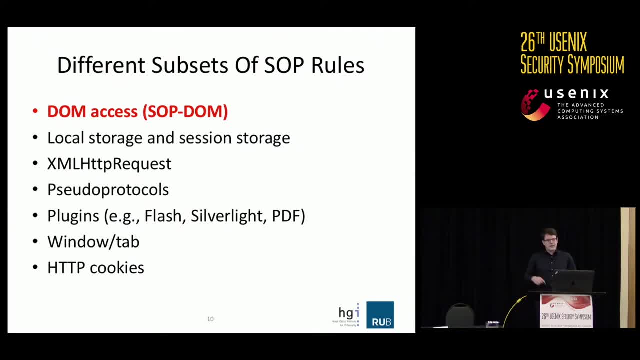 maybe the most popular example on the slide is the cookie example, because a when you compare cookies, you have to compare another factor, so not only the port and the domain and protocol or schema, you also have to consider the path. so each aspect has its own SOP and what we did is in case of the DOM SOP. 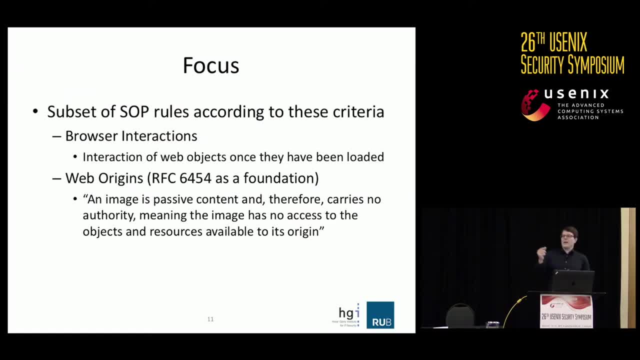 that we considered resources once they have been loaded. so imagine the case that you go on bankcom and there is an image. this image will be loaded and after it is loaded we check whether it can get access to the website of bankcom. so there might be script and an image which is possible when you look on. yeah, 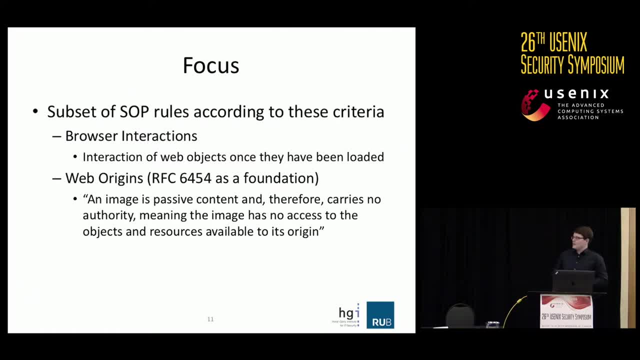 searching files, searching content files, and well, this is somehow complicated. what we also did is that we considered the RFC6454 from Adam Bath. here's just a small quote of his RFC. just read it: an image is passive content and therefore carries no authority, meaning the image has no access to the 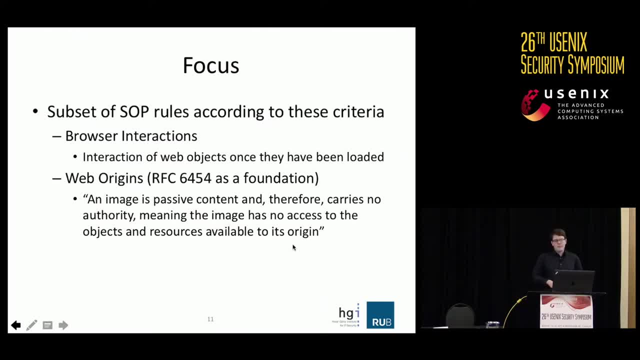 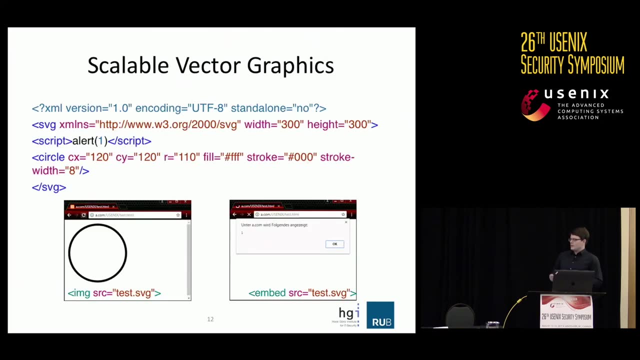 object and resources available to its origin, which means for me that an image is actually not able to execute active code because it's somehow passive. right in 2011, at the CCS conference, there are some guys, including Mario Heiderich, who published a paper about SVGs and they wrote there that 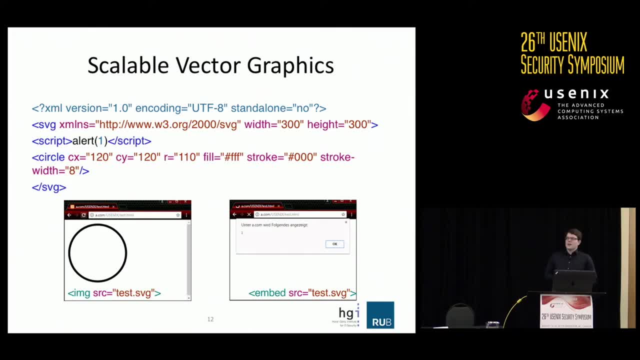 SVGs, which are actually images or scalable vector graphics, can include JavaScript code and this JavaScript code can look like this one. so we have an SVG element, we have a script element inside of that in the SVG and an alert as a proof of concept, a circle, just to show that. 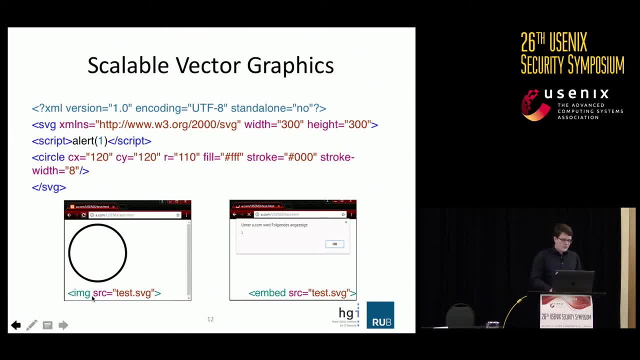 there is something in there and when we use the image element, for example in the newest Chrome, and we see that the circle will be displayed here, so we don't have the alert one window. but when we use the embed element here or object, yeah, we have a script execution, so dependent on the HTML. 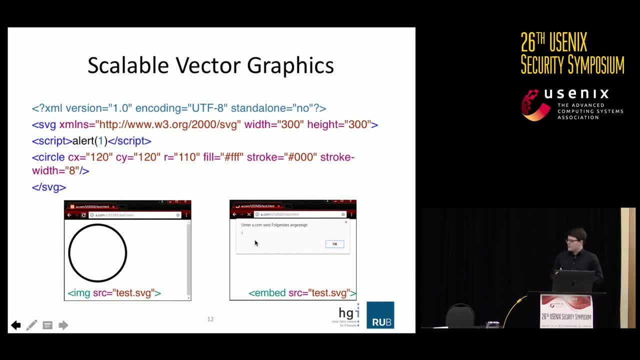 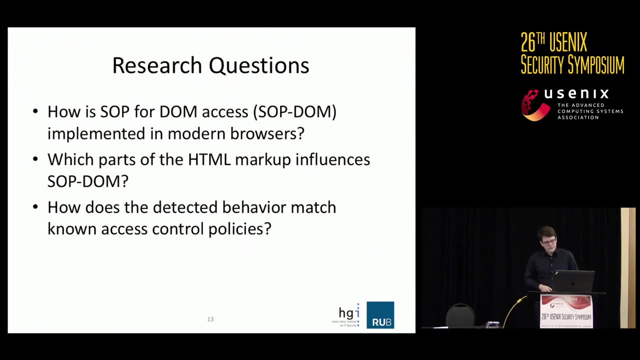 element. the browser allows you to execute JavaScript, so obviously we have a huge impact on the embedding element, which is, in this case, image or embed. so the RSC might not match exactly, so that depends always on the view, but it's totally important that we have that and we ask ourselves well which research questions might be interesting and 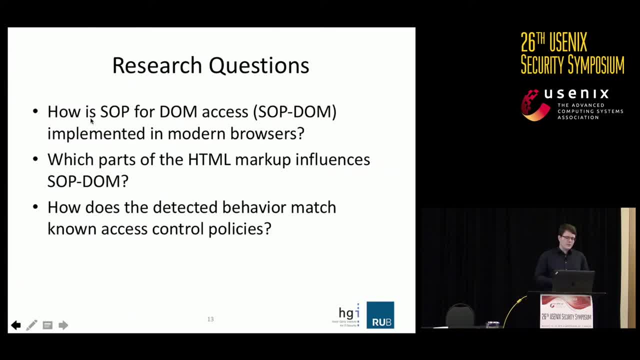 here they are. so three of them. how is the SOP for DOM access implemented in modern browsers? so what is the current situation? Dom? so we saw that the embedding element is definitely a very important aspect. so the element which loads your resource is very, very important. and third, how does the detected behavior match? 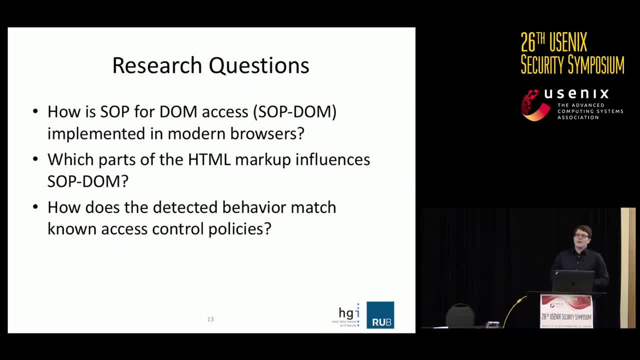 known Excel control policies. so we thought: well, wouldn't it make sense to have a formal model and to describe the sop with something like distributionary access control policies, withБ access control or role-based access control, because everybody knows how role-based access control models work in general, hopefully And well, we will see what the results are. 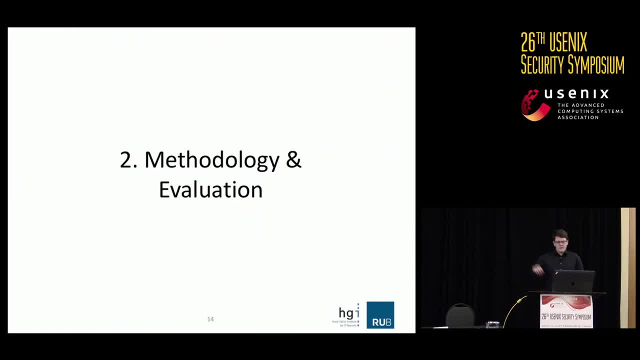 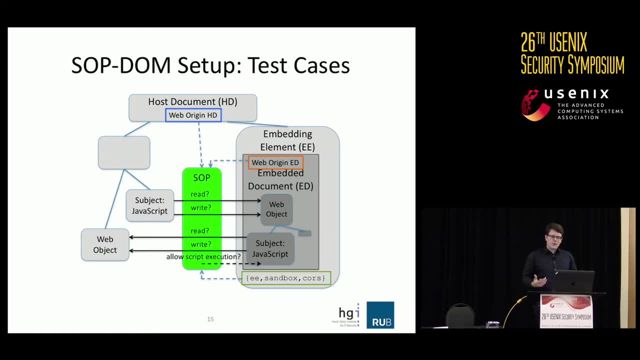 So this is my second point on the slide. This is exactly the same ordering as it is in our paper. So a methodology and evaluation. In our methodology we have such a test set up here. So in this case we have the host document, which is a browser which loads bankcom. 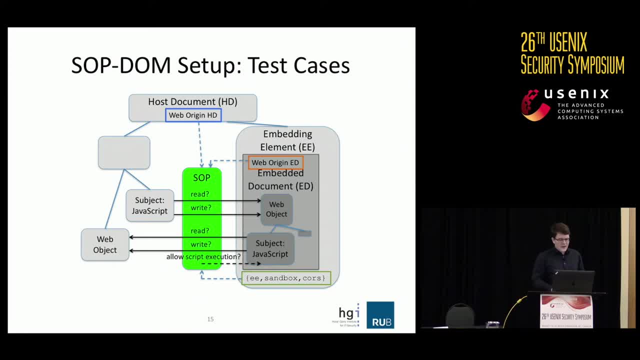 So the first example which I showed you. And then we have an embedding element. So this embedding element could be an image, an embed element, an object element or, for example, a script element or an iframe, even, And when we have a case of an iframe, an iframe. 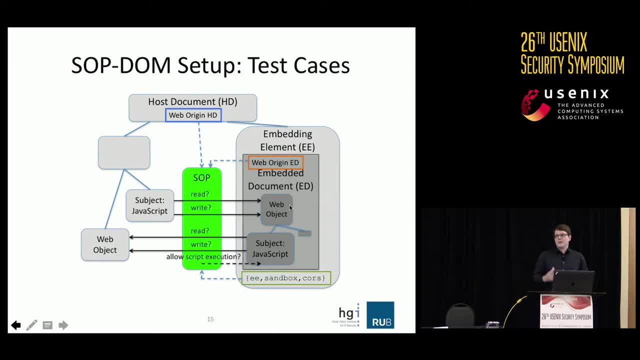 can load. And then we have another website, another subdom, And this website is here listed with the embedded document. So we have the iframe which loads content and this content is called the embedding document content. And when we look on the host document, so the first website and the included website. 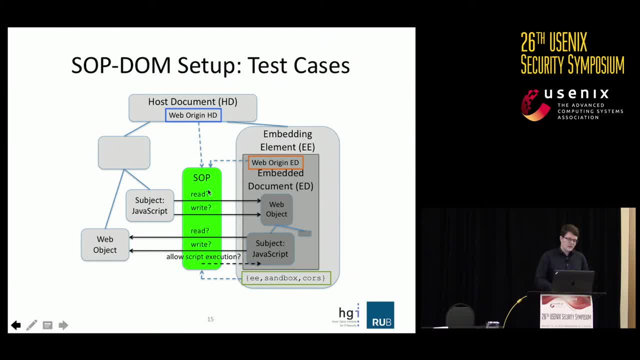 the embedded document we see that there is something like a firewall which manages the access model, access control. So, for example, when we have JavaScript code on the bankcom scenario, we might have read access on HTML code or actually the DOM API of the iframe's website, which is also bankcom And the other. 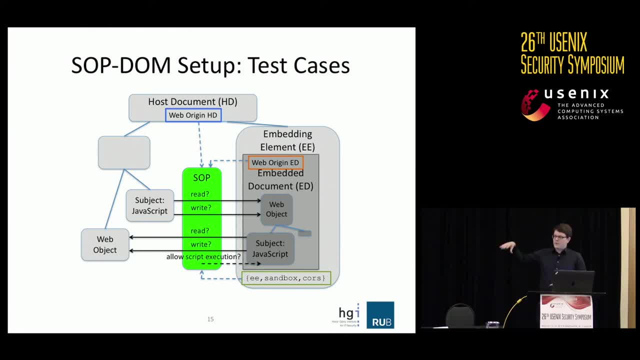 way around. when we have website from loaded in the iframe, then there might be some access methods to, for example, we have to communicate with the host document's website. So we have both directions here, which is totally fine, And we even have a next-to-read-and-write access. Also, the allows script execution method. So what this means is that you maybe know, iframes, for example, have a sandbox attribute And the sandbox attribute allows us to, for example, deny the execution of JavaScript code to use a program. So, for example, what this means is that HIFRAMES, FOR EXAMPLE, 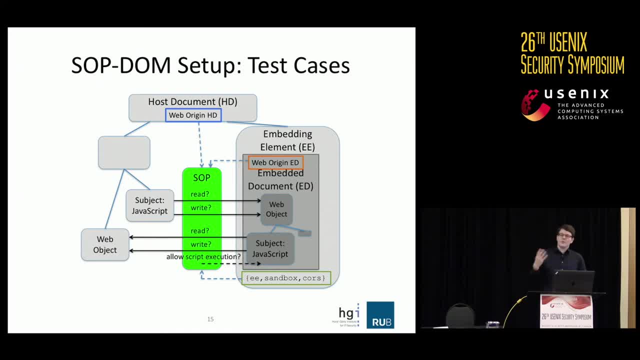 make the origin a random origin, hopefully, and some other aspects So we can influence, by setting the sandbox attribute, the whole DOM. you know, so at least parts of the DOM, And what we also see here is that the SOP. 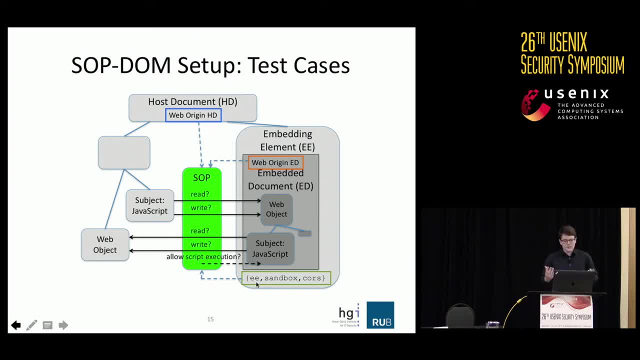 is obviously influenced by a few factors which we considered. So, first of all, the embedding element. I told you that Image versus embed, for example, Sandbox and cores, So cross-original resource sharing. We considered cores because, from our point of view, 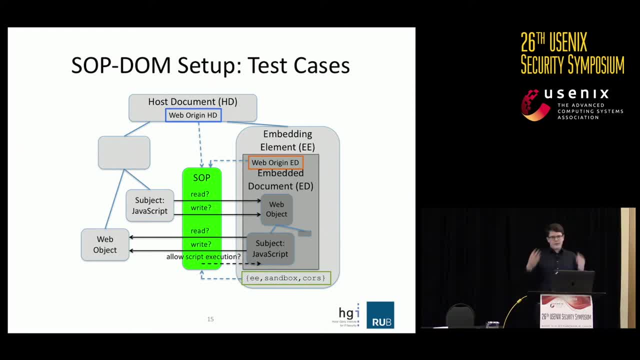 we also have a startup. There are many, many customers who use cores and they make it totally wrong, So they have a wrong configuration and it's actually a little bit complex, And you will see that this complexity leads to a lot. 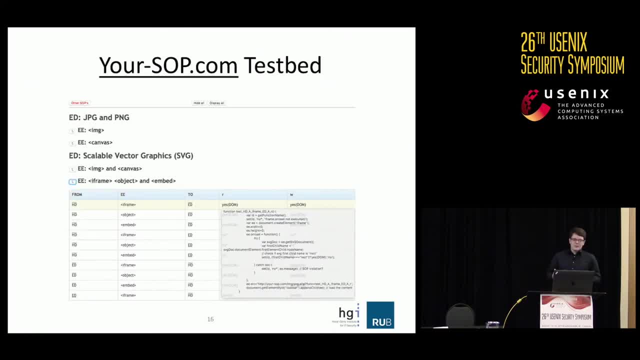 A lot of bugs, So we built a test tool which is available online via yourSOPcom. I go into my Google Chrome here Full screen, And so, as I told you, yourSOPcom, And we see that there are different test cases. 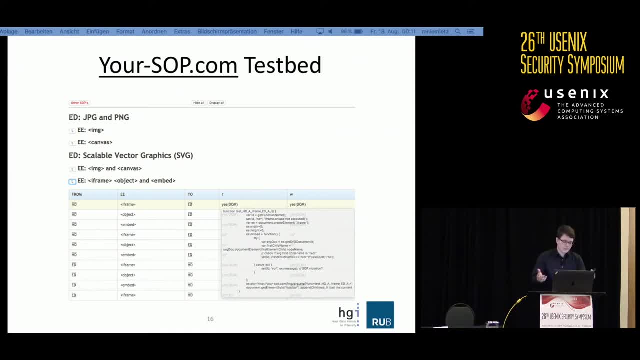 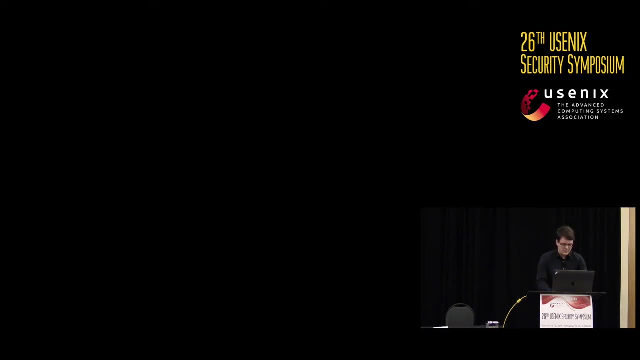 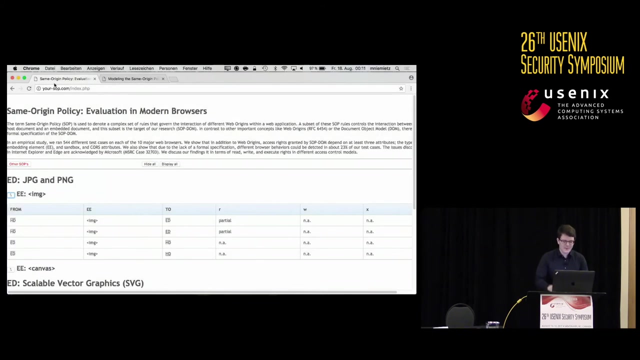 And when we click on this button here, there will be evaluated right after we click, how we R, isn't it? What do you mean? Oh, okay, interesting. Okay, then this way here, Perfect, So this is our website. 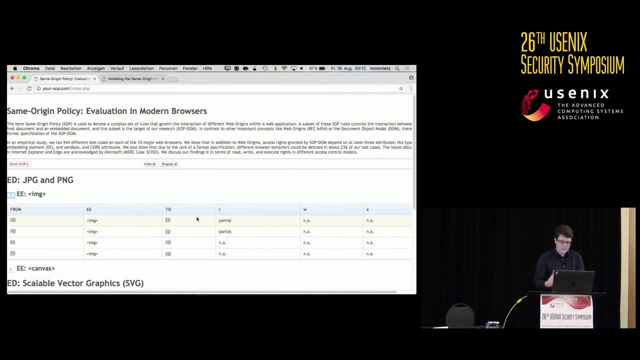 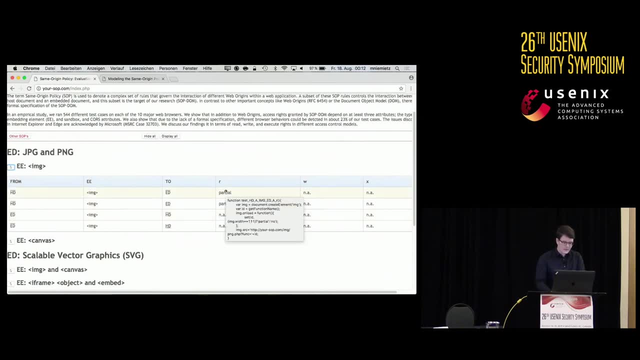 And when we click on this button here, our test cases will be evaluated right after we click And what we see is, for example, that we have partial read access in case that we have the same origins when we use the image elements. So there are different elements considered. 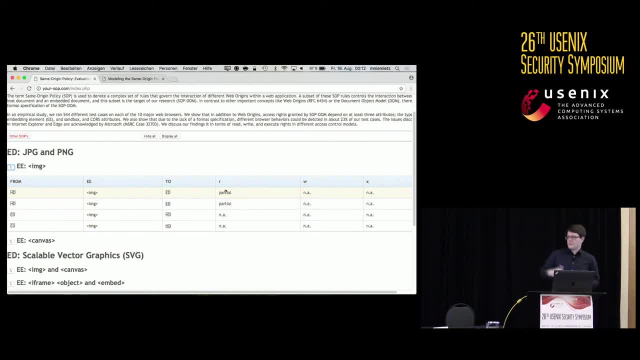 There are different origins considered, So at one time the same origin case, then other origins, And we go through read, write and execute. So when we go over here, for example, we see our test code, how we tested read access. 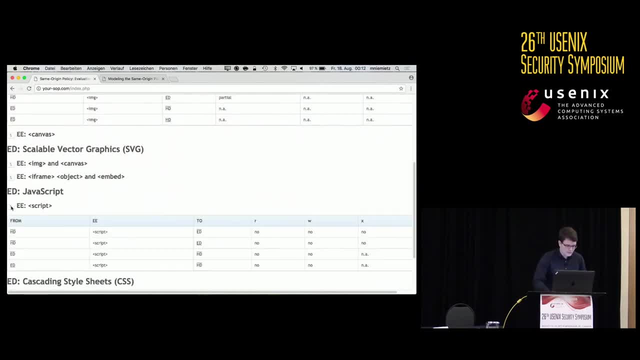 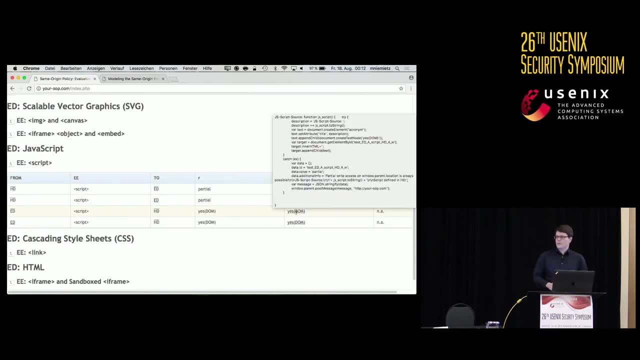 in this case. So you can check that directly. We can also click, for example, here And you'll see that we'll be directly evaluated. a lot of test cases: In total five cases: 544.. And there's another thing which might be useful. 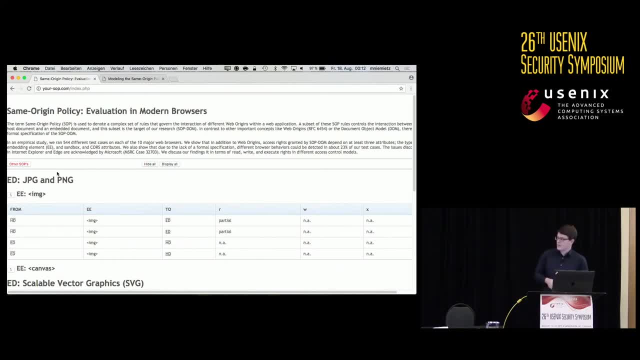 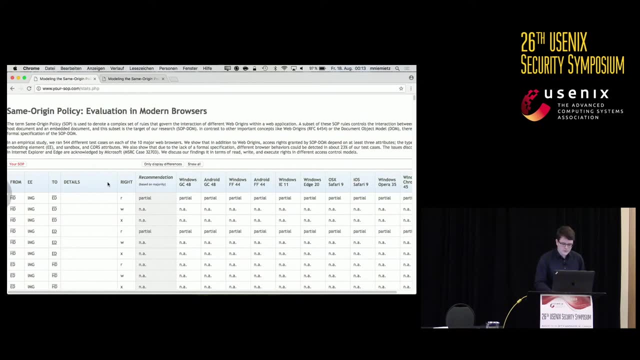 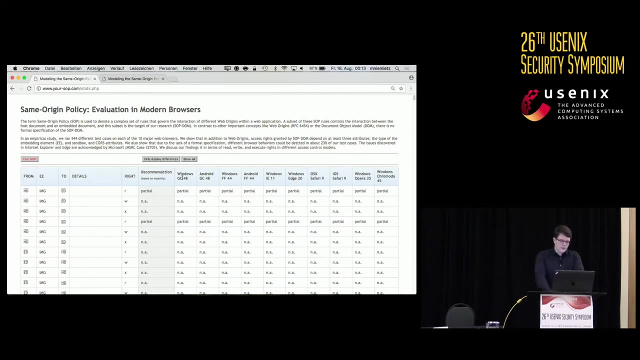 next to your own browser which you can test as a browser vendor or whatever. is this one here? So we created a test bed which compares- I'll make it a little bit smaller- different browsers, So we used Google Chrome, Firefox, IE Edge. 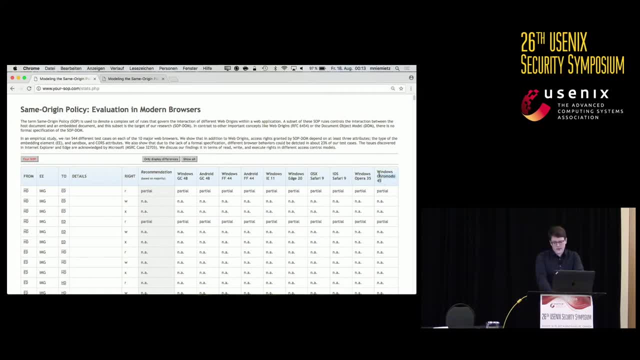 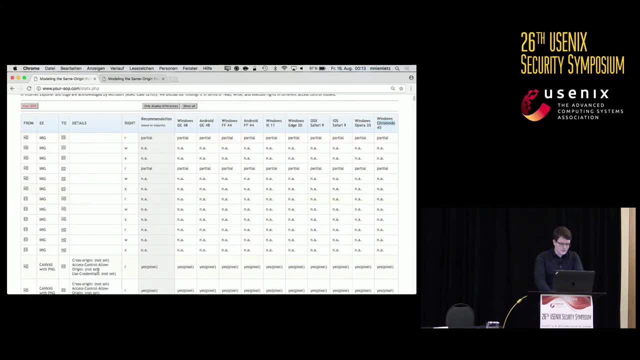 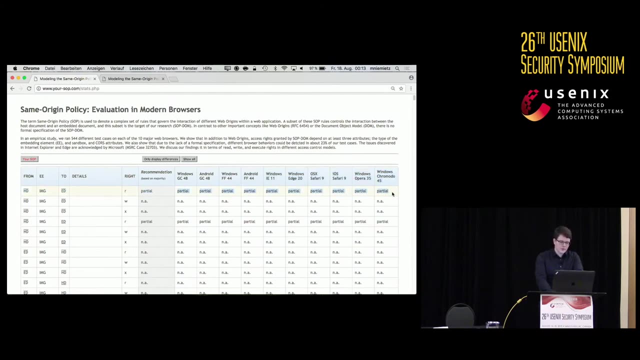 and Safari, Opera and Chrome. We actually hope that Chrome is completely broken, But indeed it is, And we see that there are different test cases And what we want is that we want to detect differences across browsers. So the first row here is an interesting for us. 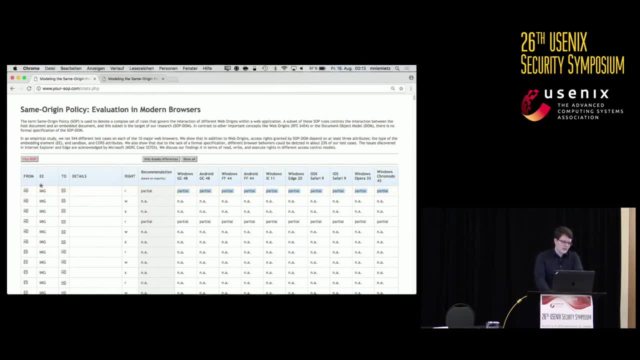 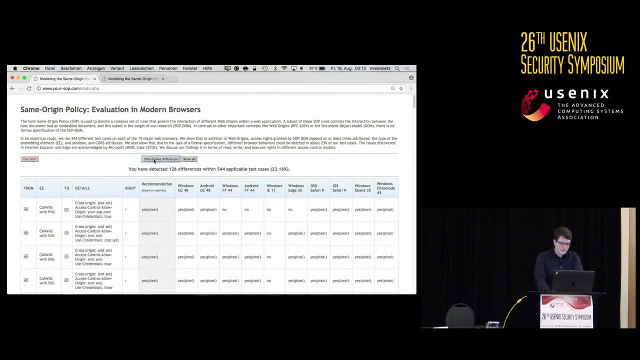 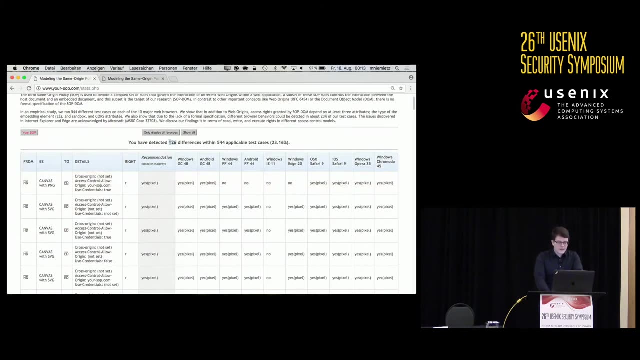 because every browser has partial read access in case of images loaded by the same origin. But when we click on the same origin, when we click on only display differences, we can see that there are a lot of differences: 126 cases from 544 cases, so over 23%. 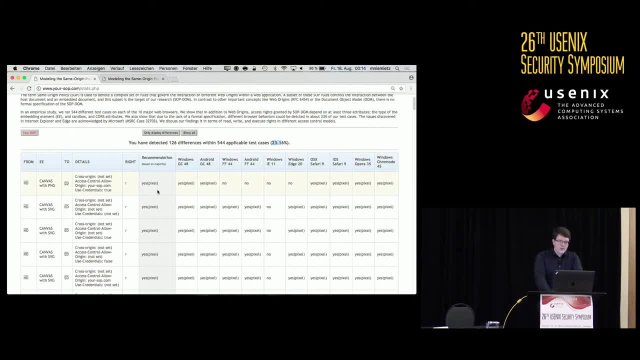 are different in at least one browser. So, for example, in this case here we can see that the recommendation based on the majority is that we have read access And most of the browsers have partial, Partial access, But in Firefox and IE and Edge we don't have access. 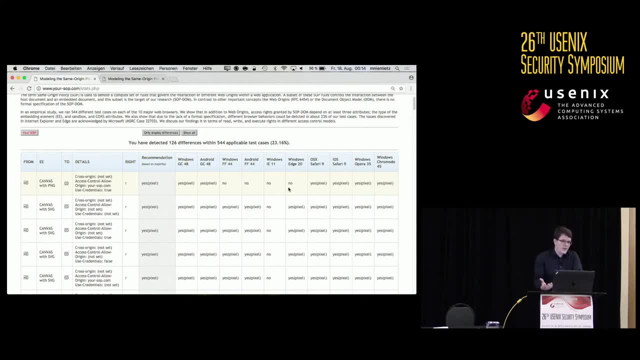 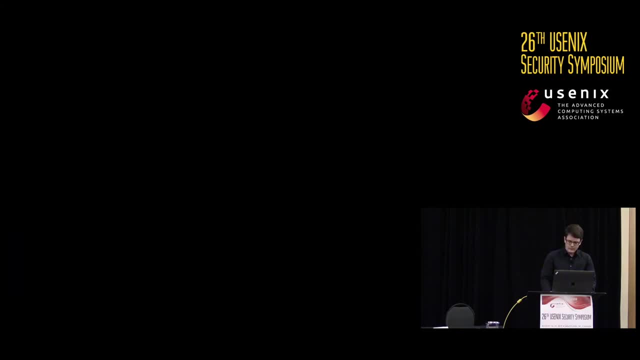 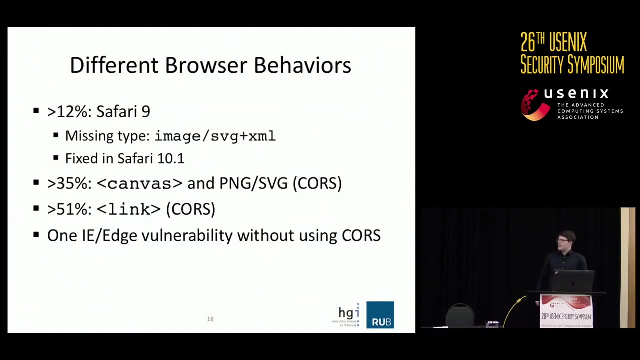 So something might be wrong here. So is this OK Or is this a bug? This is up to you. So let's go to the presentation part. So what we did is that, after creating our tool, is that we categorized our browser differences. 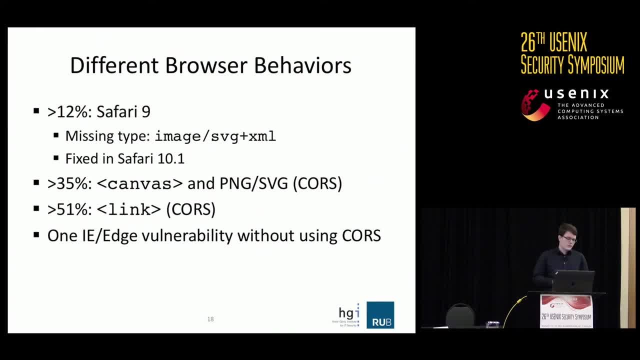 And, First of all, we saw that over 12% of the test cases were different because of a bug in Safari 9.. So what we- yeah, it might be all- missed is that we didn't use image SVG plus XML as the content type. 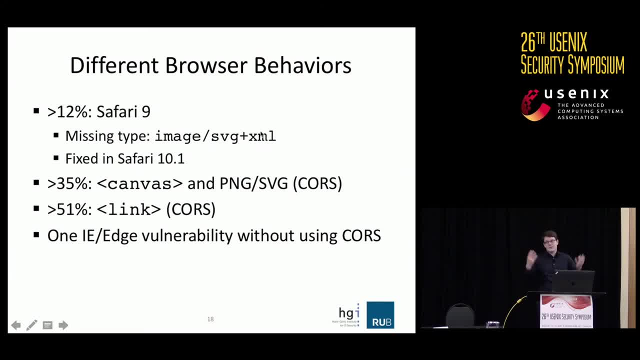 But Safari 9 required that, though it wasn't standardized in the W3C standards or what WG OK, And this behavior was fixed in Safari 10.1. So it was maybe obviously a Safari bug, And this is a little bit more interesting. 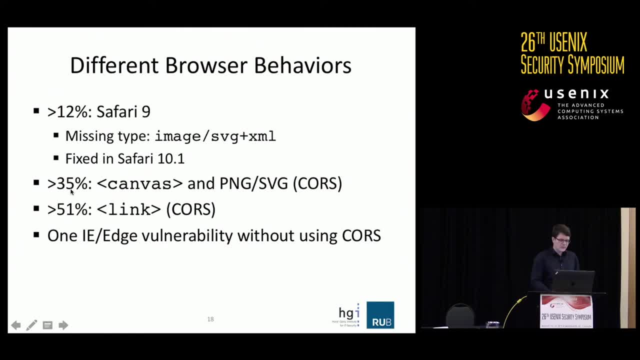 Over 35% of the test cases were caused in case of canvas elements. So we tested the most- yeah, let me say used and well-known elements like link, script and frame, And this also includes canvas, because you can, for example, 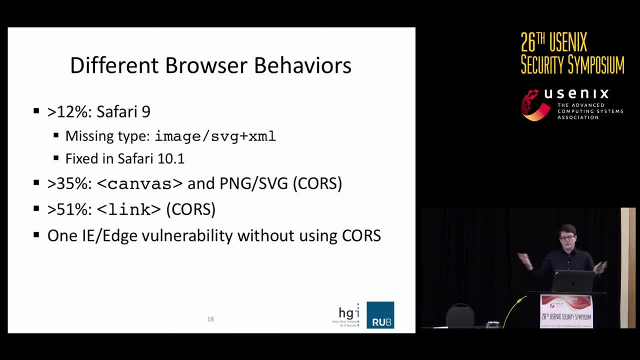 communicate with image elements, which we also tested. So this is actually related to it And we see that canvas loading content- and this content is PNG or SVG in combination with course- have a lot of differences. Also links. So when we load CSS code with it, there is a lot of differences. 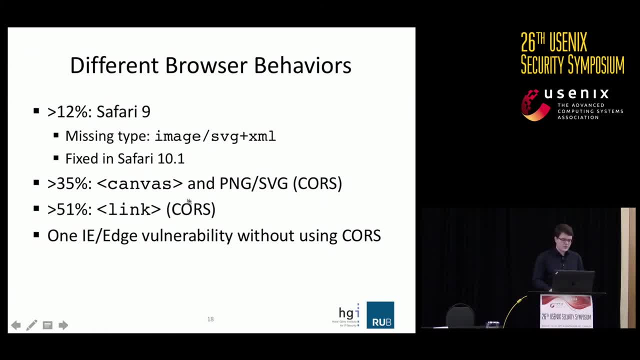 Over 60, 70%. There are 70 differences just because of the link element in combination with course. So course is obviously a huge problem. When we count them together, we are over 86% of our test cases who have problems with course due to its complexity, I think. 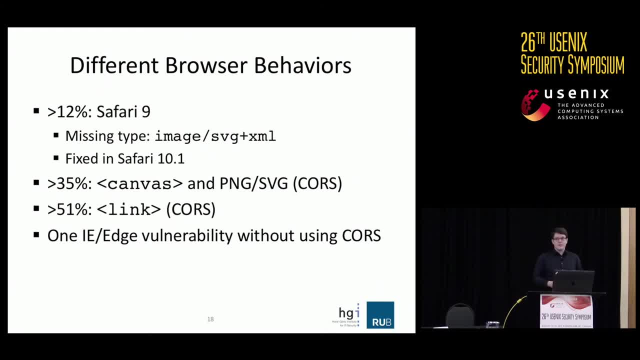 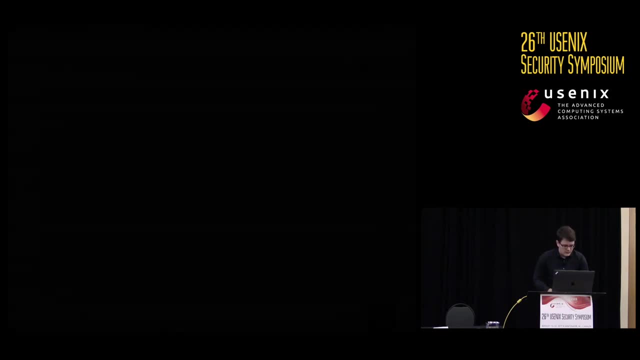 We also detected one browser vulnerability. There might be even more browser vulnerabilities in our test, but we were not able to detect them. You can look through it. Maybe you'll find one. And well, Let's go through it. So let me check here on the tool. 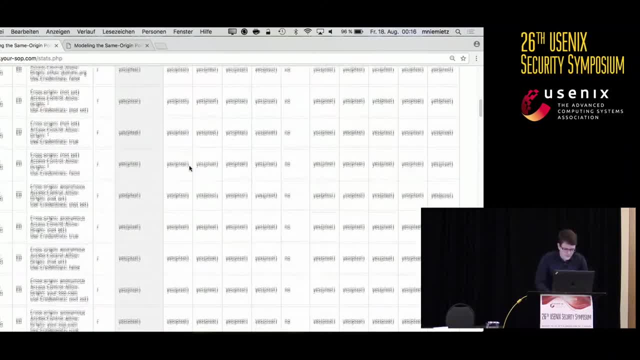 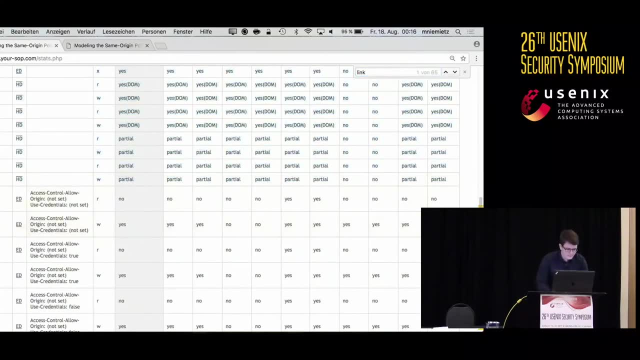 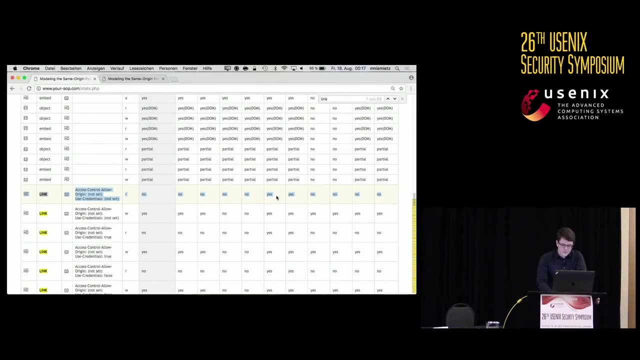 So we once again go to the tool here And the interesting line is links. So I look for it And we see that this one here might be interesting, Because every browser denies access And the only browsers, so the site of two browsers. 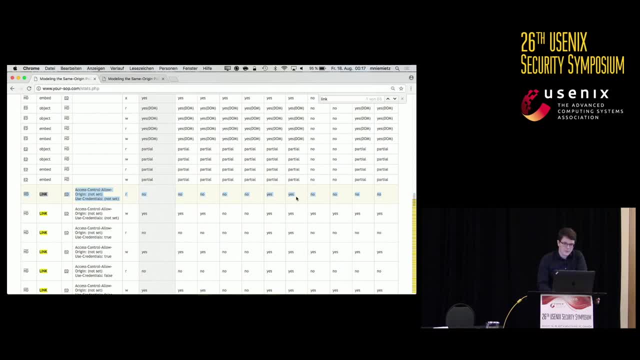 and the only browsers who allow access, the only browsers who allow access are IE and Edge, so the Microsoft browsers. And we ask ourselves: well, why is it the case, And what kind of test case is it? So when we go through it, we have different origins. 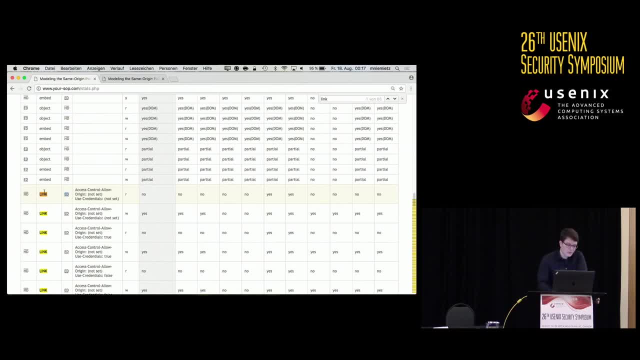 So not the same origin case. We have the cross origin case. We are using the link element We don't use course. This is not set And we have a read situation, So we want to read CSS code from another origin. This shouldn't be possible, right? 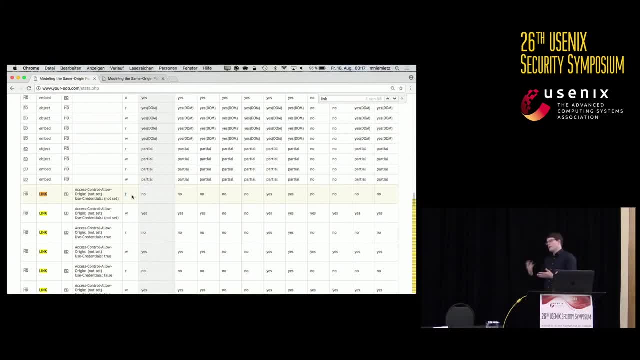 Because when we can do that, we could, for example, make a lock in Oracle Who knows? And the other way around. we can not only read code, we can also write code, cross origin, Which means that we can, for example, 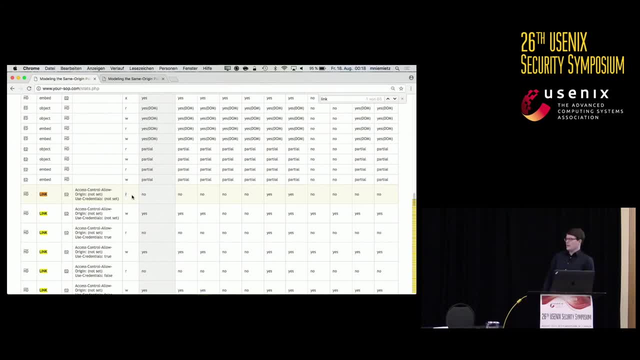 do scriptless attacks, which we announced in 2012 at CCS. So scriptless attacks- for you who maybe don't know it- are attacks which are With CSS code and sometimes similar to cross-site scripting, So you have some parts which act similar. 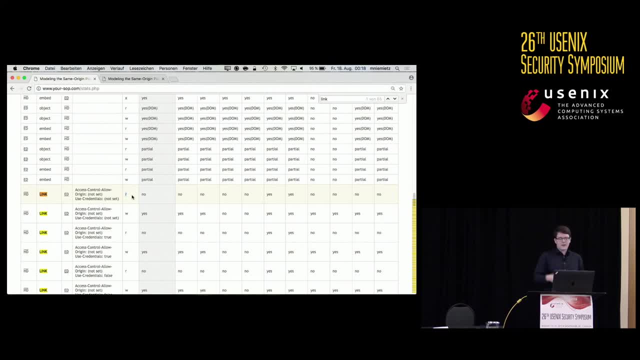 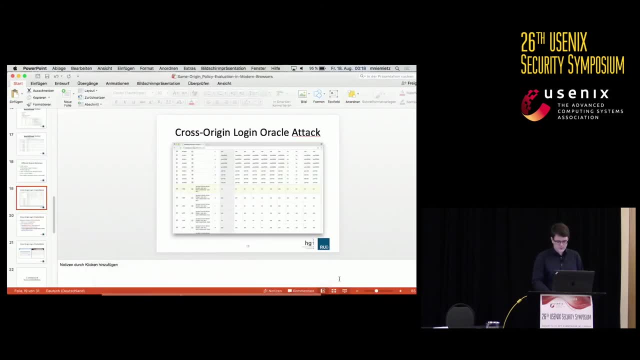 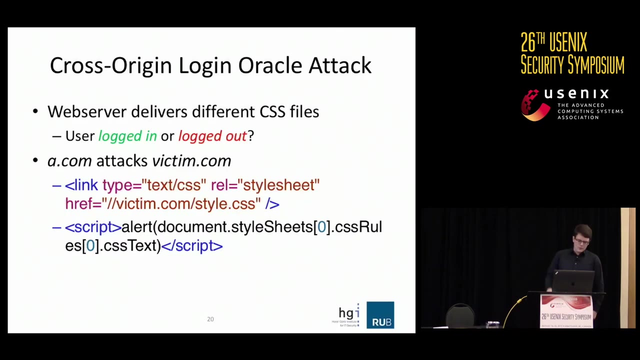 So there is a huge impact by writing and reading CSS code. CSS lines cross origin. OK, So here's an example how we can use this bug. So imagine the following case: You are visiting a website, for example startpageme. 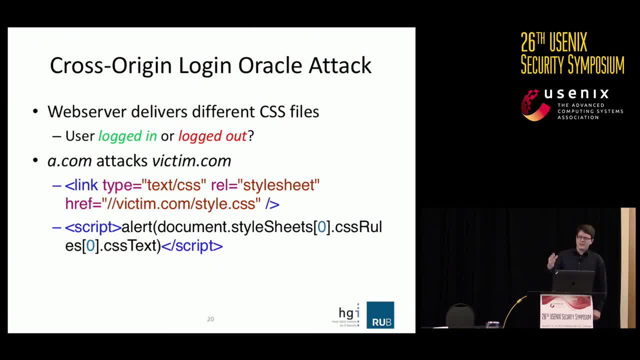 I think the bug is still there And what you see is that, depending on your log in state, the CSS file will change its content. So when we look, for example, in the first line of this website, we see that the button is displayed in green. 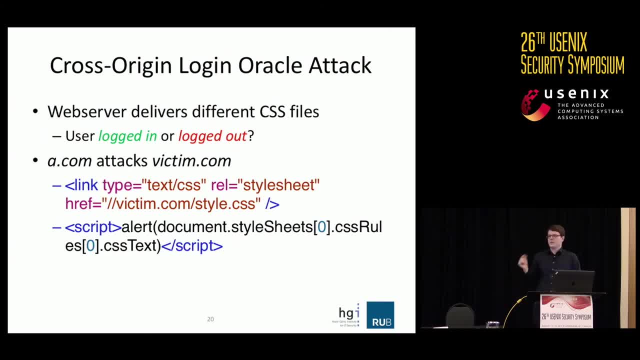 when you're logged in And when you're logged out, the button is displayed in red. So the CSS code, the CSS file, changes It's content depending on your log in state, And we know from our tool that we can read out. 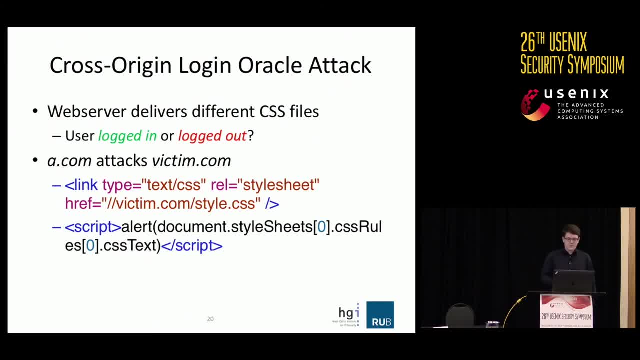 the CSS lines cross origin. So, for example, with this proof of concept here, an alert window with document style sheets 0.. So the first style sheet, CSS rules 0, CSS text. So we read the first line of the loaded CSS file. 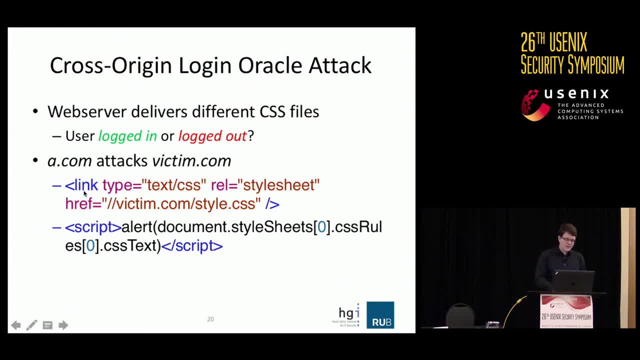 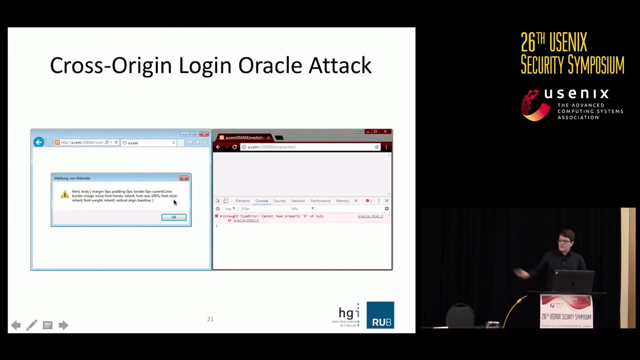 And how can we do that? Just by including a link element on our host document website, on our attackers website, which loads the attackable CSS file, So, for example, from victimcom or startpageme. So this is the result in IE on the left side. 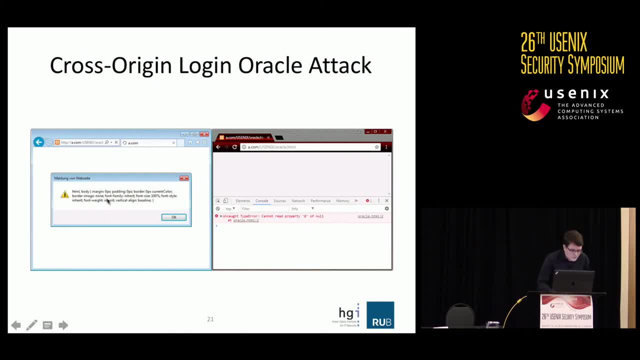 and on the right side in Google Chrome IE, as you can maybe see, it reads out the line perfectly and shows it in the alert window, And this is just a POC. And on the right side we have an exception here. 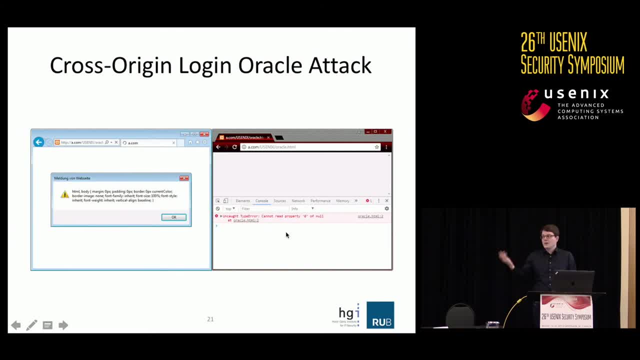 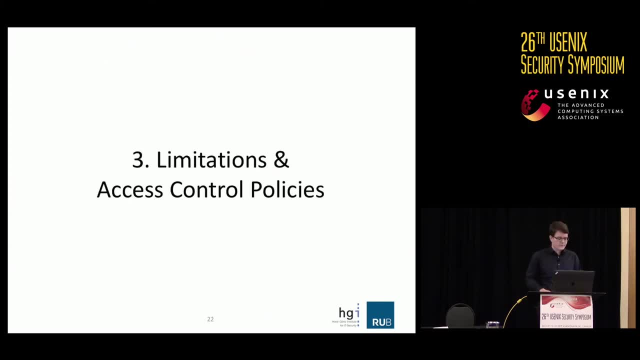 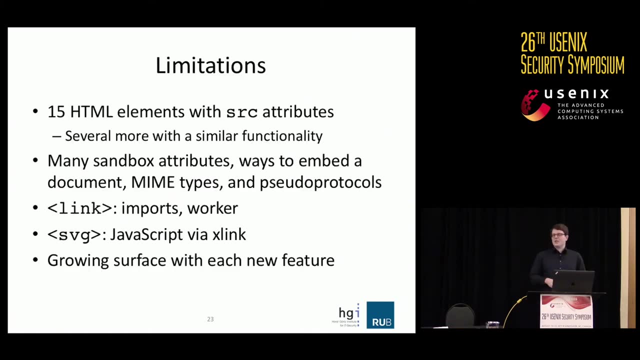 And Google Chrome denies access, So we cannot read out the CSS code with its browser, which is actually the right decision. So limitations on access control policies: There are actually a lot of limitations. We had a look on a few elements, On some origin aspects, so we only considered HTTP. 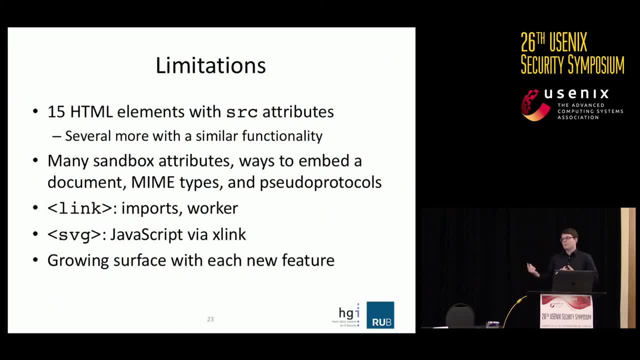 We considered different domains, not different ports, and many, many other things. So when you look on the limitations, you can even write a book about them. So, for example, you have limitations in case of link elements. There are CSS imports. 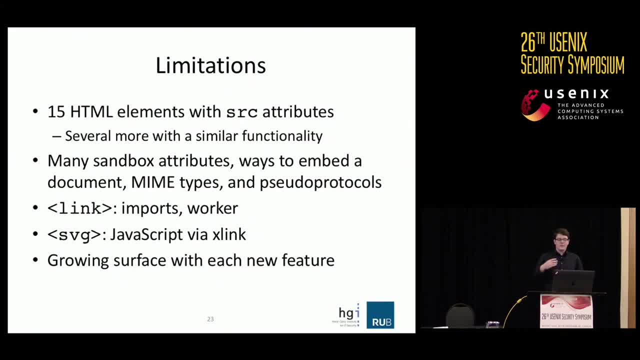 There are web workers, service workers. We have SVG content, JavaScript execution inside of the SVG via X-link and many, many more things, Pseudo protocols. You can even define your own pseudo protocol, So if it's, for example, possible to define burger colon, 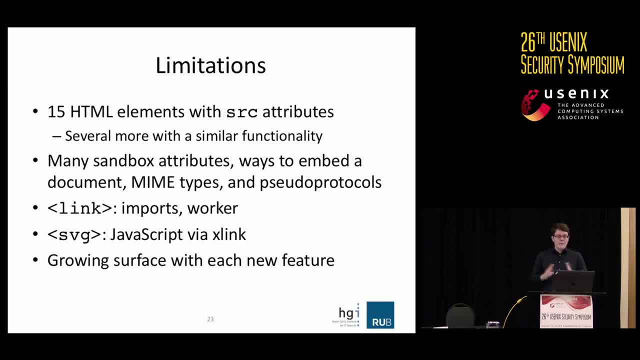 as a pseudo protocol- And this is a totally new area and might have also some new SOP bugs, Who knows. And the cool thing about it, or actually worse thing about it, is that the attack surface, The attack surface, might grow with each new feature. 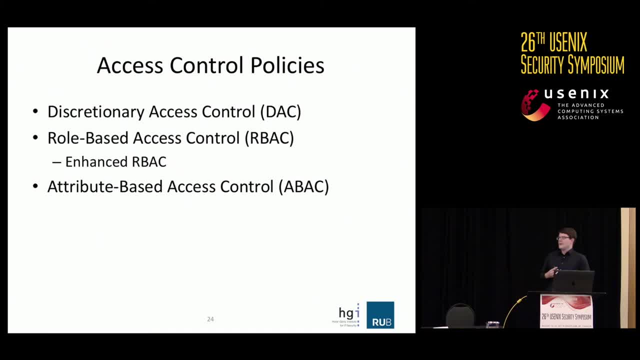 So the last part of our paper discusses different access control policies And, just to make it short, we discussed the discretionary access control model, which you maybe know from UNIX systems: Read, write, execute. Role-based access control models. We also proposed enhanced role-based access control. 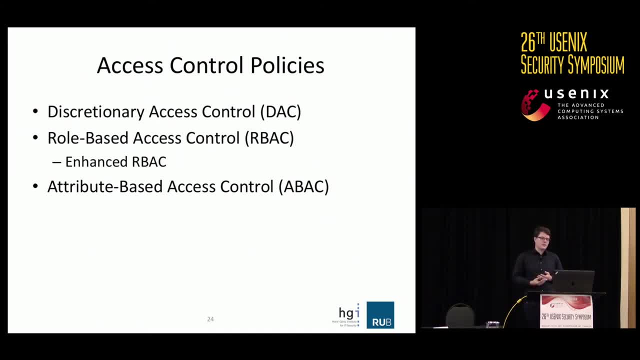 models And attribute-based access control. Yeah, we discussed it. if it could be matched to the SOP model And maybe just to give you one example, when you look on the discretionary access control model, you maybe think that because of the name, 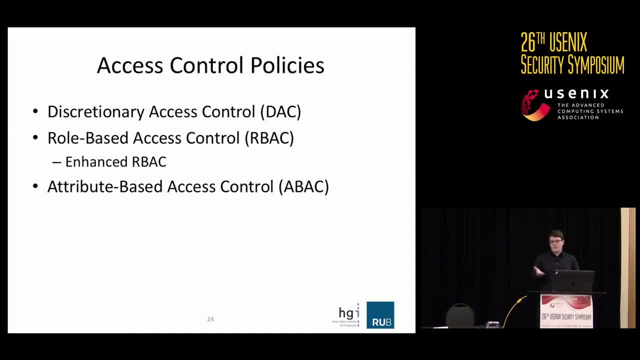 the same original policy only gives you access in case of the same original policy- case right- But obviously this is not the case when we look on script elements, Because script elements can include content from a number And you can also include content from another origin, which? 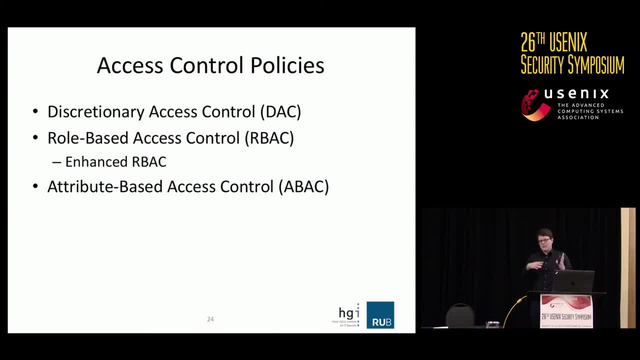 will be executed in your own origin by just including it, So you could build a matrix. You could build a discretionary access control matrix with it. But it's not really easy to do that And we might think that the role-based access control model. 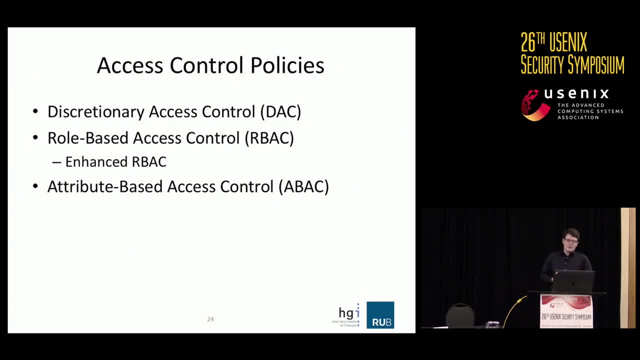 and attribute-based access control model might be a better decision, But yeah, there are many, many more aspects about it. Also, by the way, the role-based access control model, which is a very important one. The role-based access control model. 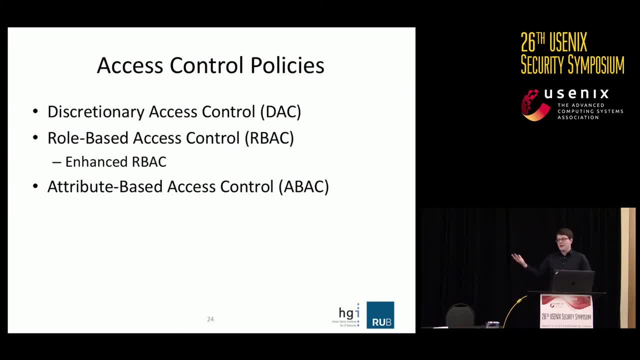 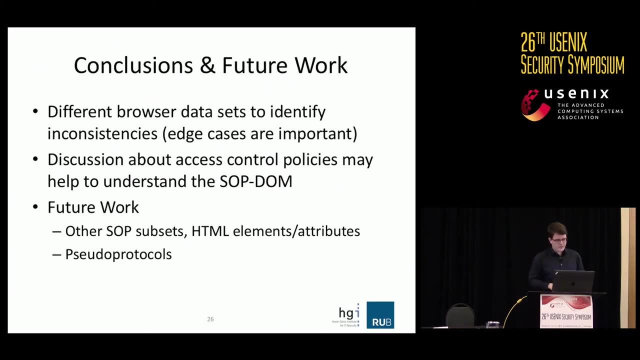 might be a good fit because we saw that the embedding element, like image or embed, is a huge factor, a very important aspect of the SOP. So conclusions and future work: There are definitely different browser data sets And we found a lot of inconsistencies- nearly 23%. 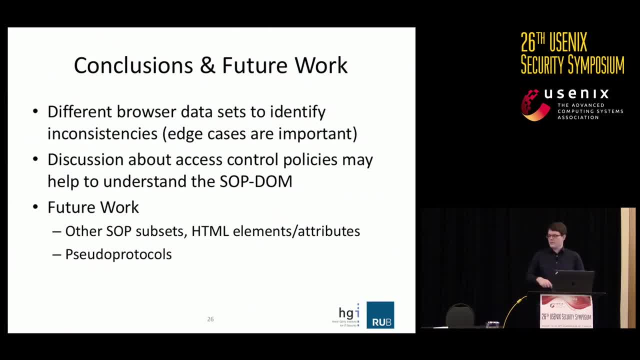 of you. We found that the test cases were different, most of them because, of course, And we can actually see that each new feature, each new browser complexity might lead to security bugs. So think about it when you introduce a new HTTP header or when you introduce a new attribute which 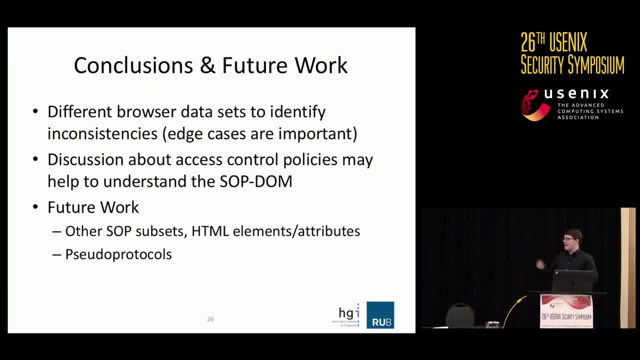 might protect you. So there will be definitely bugs And it's hard to implement them. We talked about with the W3C and WattVG guys about some test cases And even these guys don't have all test cases for the most popular elements in case, of course. 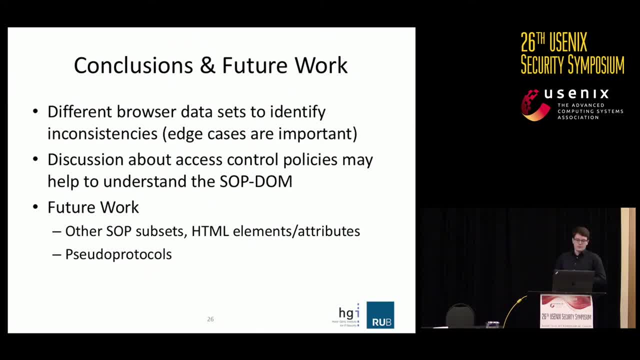 So there's a lot of things to do And, yeah, you could maybe help. Future work might be also to consider other subsets, maybe Silverlight, It might be interesting- Different pseudo protocols, data UIs, for example, and different HTML elements and attributes. 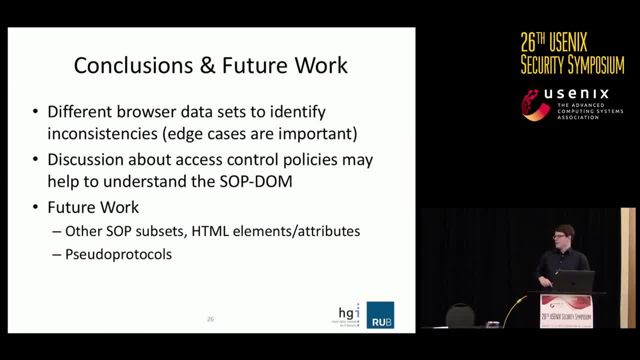 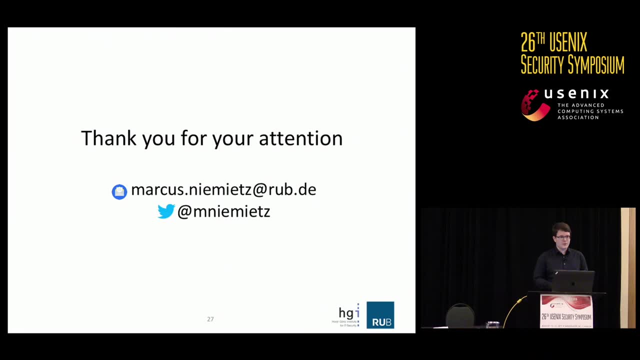 Especially when we look on HTML5 and some other new- yeah, let me say- standards, we might find new things, new features which make the situation a little bit worse. And well, I hope that you enjoyed the talk And thank you for your attention. 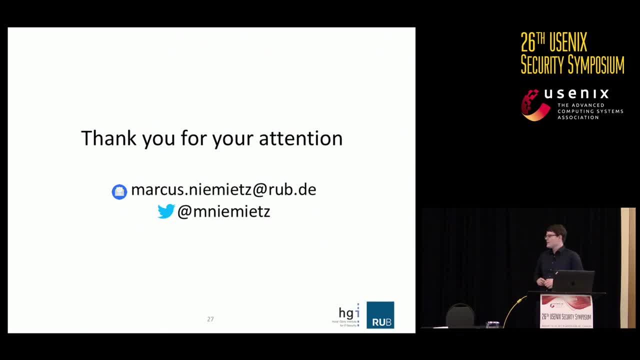 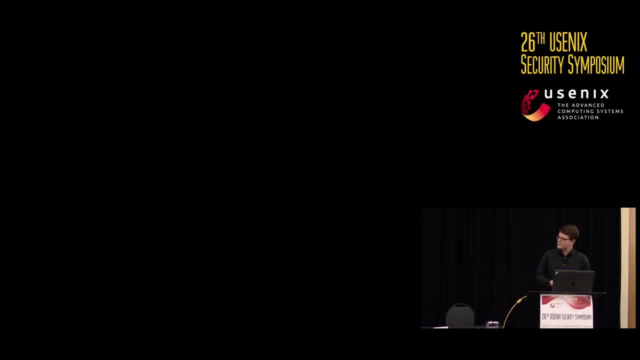 Yeah, very nice, Very good work, Also very valuable. When you display these big tables, you have this binary thing, So there's full access, no access, And then you have the partials. So what I was thinking about, did you? 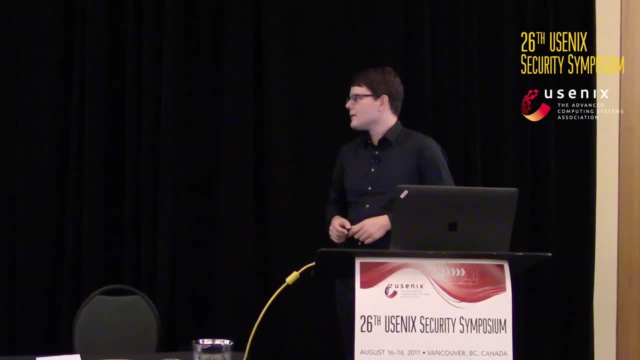 check if partial access of browser A is the same partial access as B, Or do we also have differences there? MARIUSZ GASIEWSKI- Partial access is, for example, when you test for if you can read all the pixel of an image. 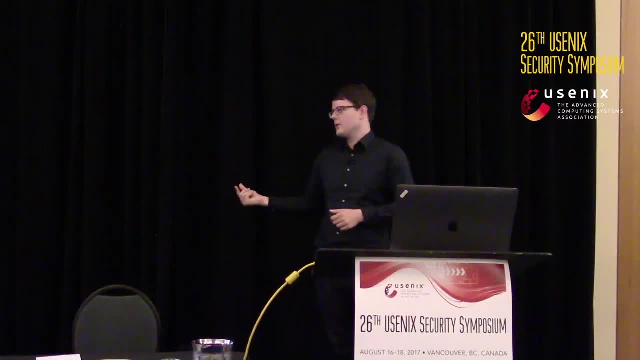 And the test case is the same when you look on the same origin or cross origin. So there's no difference in the test case. OK, so it's the same. It's not. I can. one browser can read some of the parts. 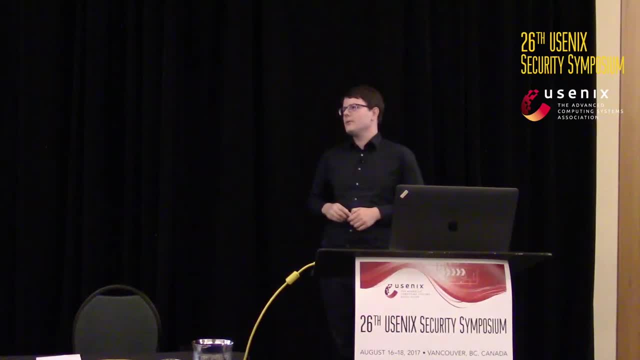 but others not. So they will check on that. MARIUSZ GASIEWSKI- Yeah, we didn't implement that, but yeah, there might. there could be some differences, OK, so future work. MARIUSZ GASIEWSKI- Good point. 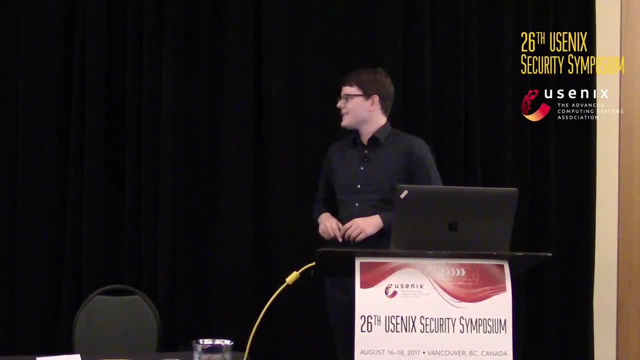 And the other thing that I was thinking about. so again, the same origin policy is much older than CORS, And CORS was introduced to give some more flexibility, But CORS comes from a time where people knew how important the web is and also how to write specification and how to proper work. 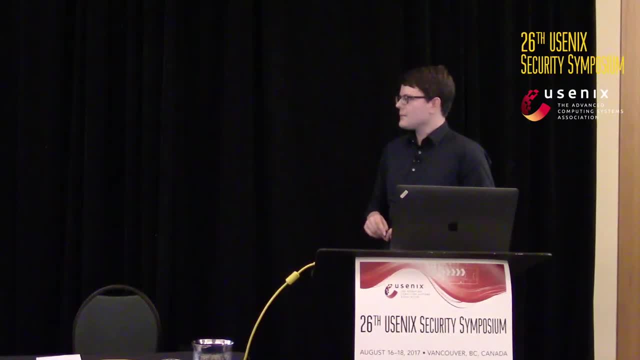 So I always thought CORS is one of the prime examples to do something right. So I'm very surprised that you find a lot of inconsistencies with CORS. So is the behavior of, or the influence that CORS has, and the behavior of the browser? is this properly documented? 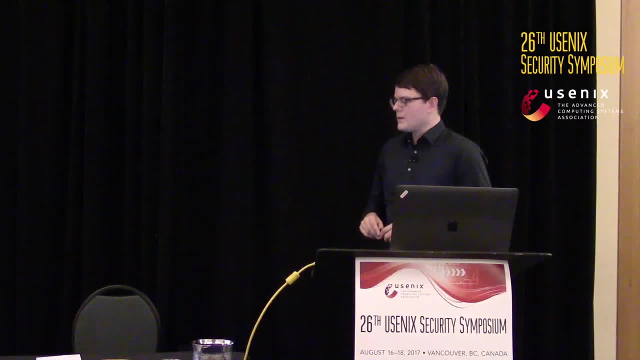 Or is this what? now the browser windows come up ad hoc. MARIUSZ GASIEWSKI- Yeah, from my personal point of view, it might be that CORS is actually too complex, And we saw that in case of CSP, right. 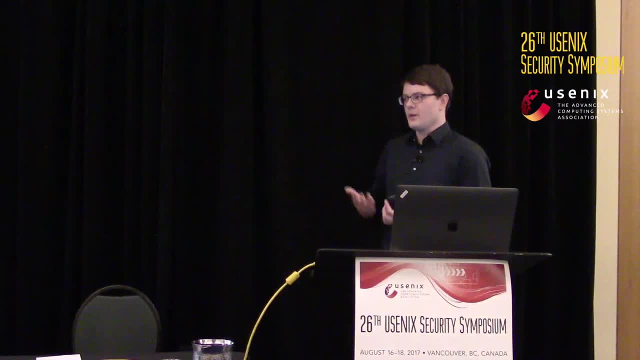 CSP 1.0 was actually very simple and there were not so many bugs. Then we had CSP 2.0, and we have 3.0, and the complexity grows. And then we have guys like Ben or you. 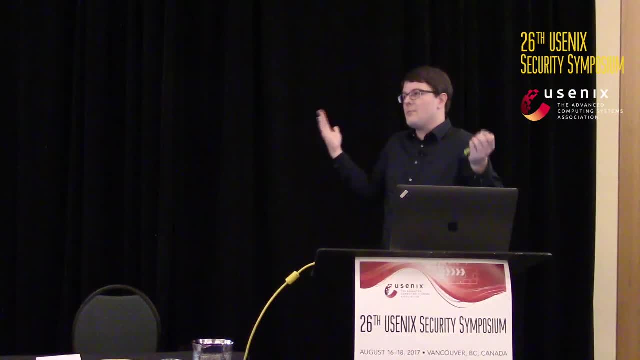 who write cool papers about the SOP and how to bypass the same original, And then we have the content: security policy. So I think that you should reduce the complexity. This is maybe the most important thing, But this is always depends on the view. 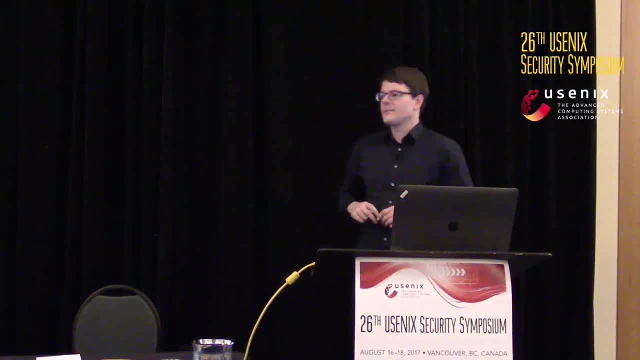 OK, so I don't have to introduce myself About the reading of CSS cross domain. So I know that, for example, like the SCAD, computed style was kind of changed such that you can't do history anymore, But I'm wondering if you cannot actually use side channels. 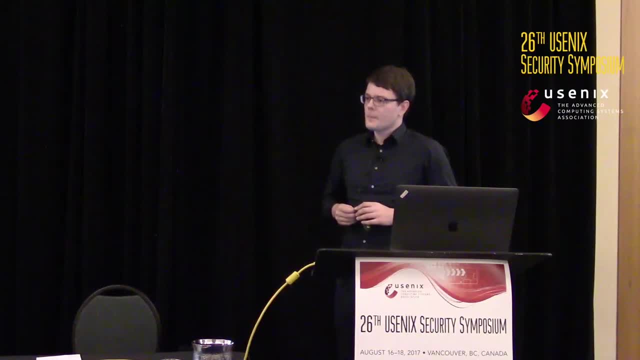 Like, for example, if you MARIUSZ GASIEWSKI- Yeah, I don't know that the font size is specified And you see basically where the next element after the text is. And did you also consider that in your test bed? 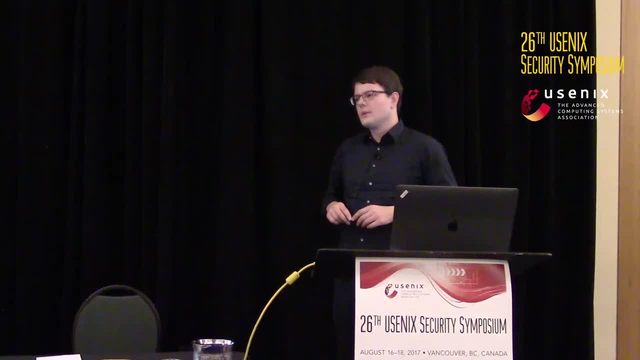 Like these side channel kind of things you can do. MARIUSZ GASIEWSKI- No, no, We didn't test that. We discussed that in our CCS paper in 2012 with scriptless attacks, but not in this case. 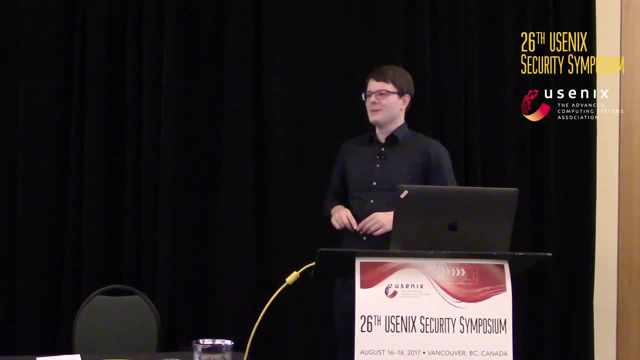 So it took a lot of time to implement these test cases, believe me. So a lot of them. Thanks, MARIUSZ GASIEWSKI- OK, So yeah, thanks again, Markus. MARIUSZ GASIEWSKI- Yeah, thanks. Thanks.